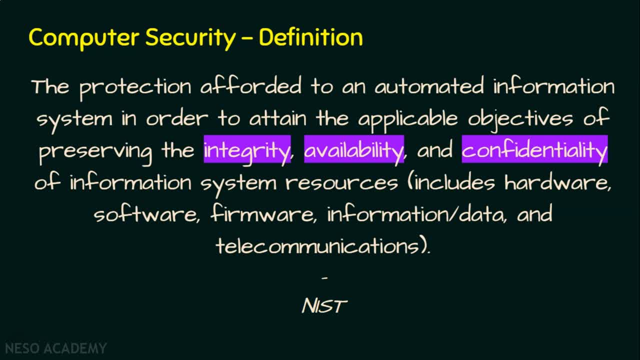 Ultimately, we are going to provide security to the system. The system includes both hardware and software. Not only hardware and software. we should also focus on the firmwares, or the data or the information that is processed by the system, And not only this: the telecommunications as well. What is telecommunications? 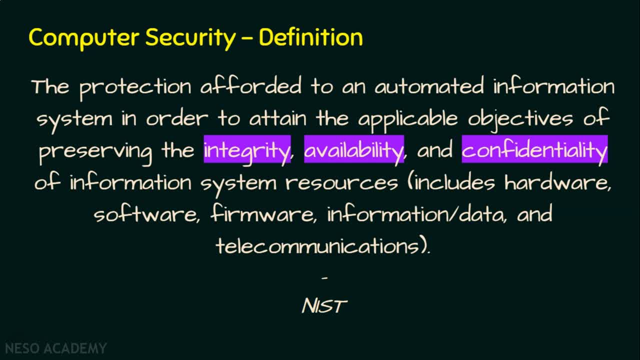 It is the communication at a distance. So in this subject we are going to focus on security in all aspects of the computer networks, And obviously computer networks has a lot of things to deal with If these three key objectives are clear, ie the integrity, availability and confidentiality. 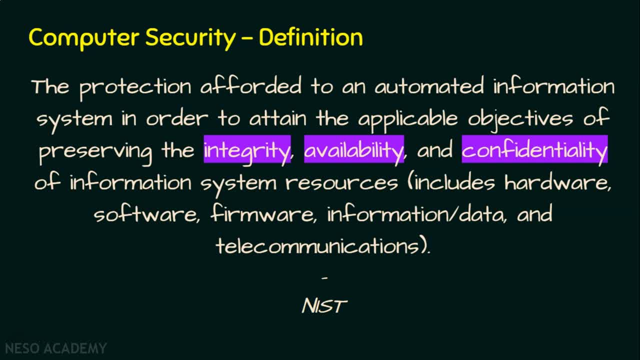 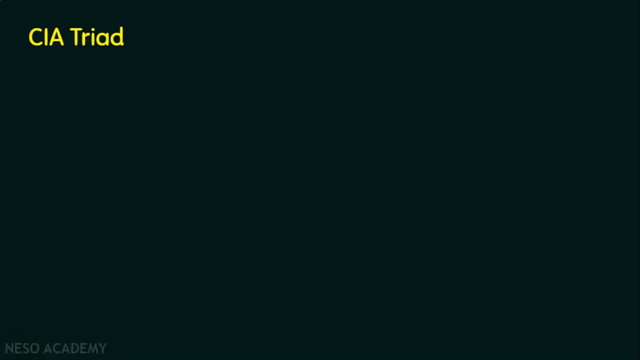 then the definition will be clear. Anyway, we are going to see these three key terms elaborately in the CIA triad part. Let's now step into the CIA triad. What is the CIA triad? The name itself says it itself says that it is a triad. Tri means three, So there are 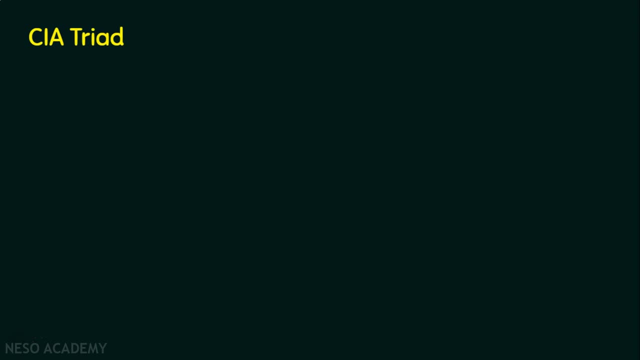 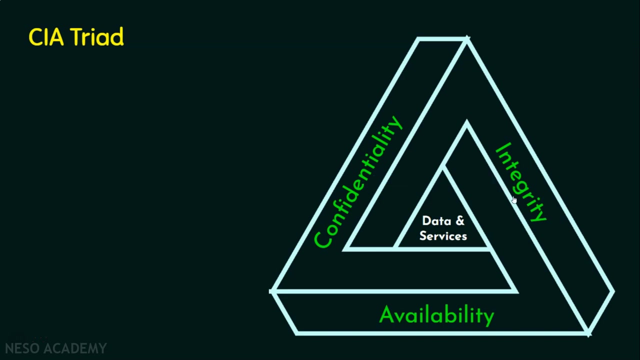 three key elements of this CIA triad. Let's see what are the three key elements We can see. the first element is the confidentiality, the second one is the integrity and the third one is the availability, And we can notice that everything is for the data and the services we are going to do with the 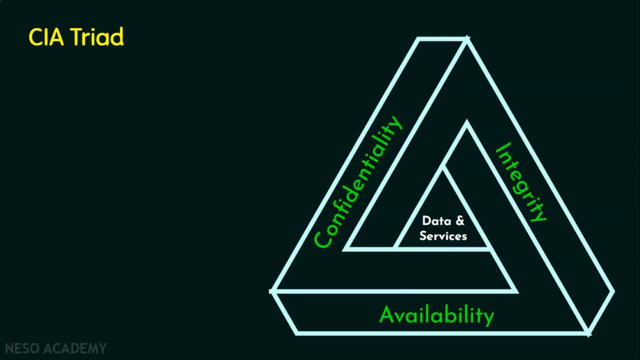 computer system. Alright, let's see the key terms elaborately. Firstly, we will focus on the first key element, the confidentiality. When we say something is confidential, what do you mean by that? It means others should not understand, except the parties who are involved in that transaction. 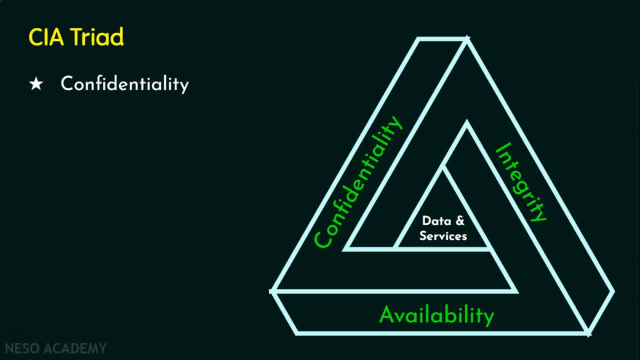 Say, if I am drafting a letter to my friend and if I mention that it is confidential, this confidential message means it should be known to me as well as to my friend, right? Because these two parties are legitimate parties involved in this transaction. Now, if an anonymous person receives this, 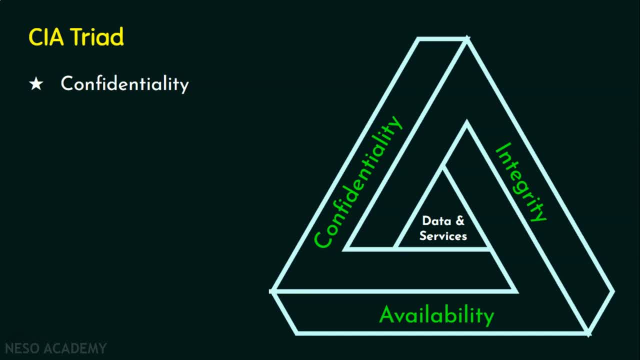 letter or message and if he sees the message or the content- what is there in the transaction- then ultimately there is loss of privacy, right? So obviously we don't have any confidentiality when somebody sees the message. So we need to prevent. 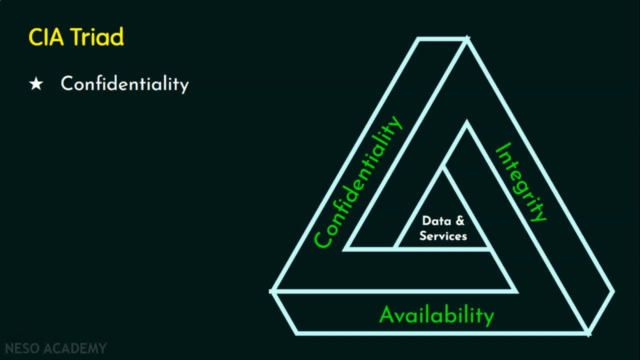 unauthorized access and disclosure. Unauthorized access means nobody else can access except the right entities who are involved in the transaction, And disclosure means the message should not be open enough To be simple. if the message is encrypted, no one else can see what is the message except the 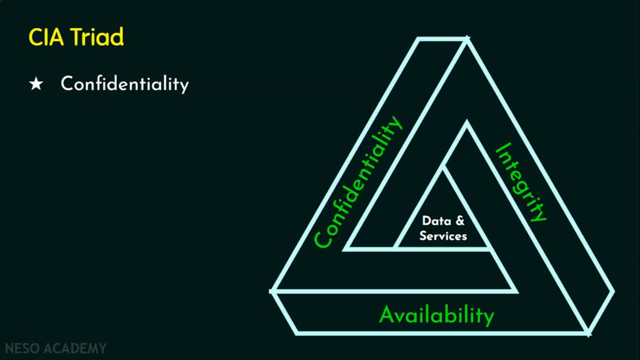 sender and the receiver. right, Because the sender and the receiver only will know what is the message, what is the key, what is the encryption algorithm? everything right. Generally, encryption algorithms are kept public and keys only are kept secret. Anyway, I will. 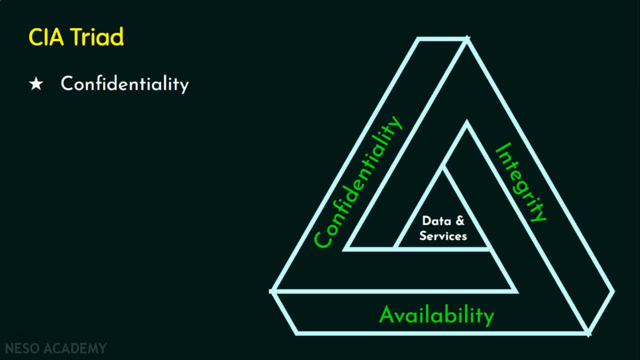 talk about this later. For time being, just understand. confidentiality means we need to protect the data that is being transmitted. If it is encrypted, obviously it provides confidentiality because no one else can see what it is right. It is a scrambled text that they are seeing, No one else should. 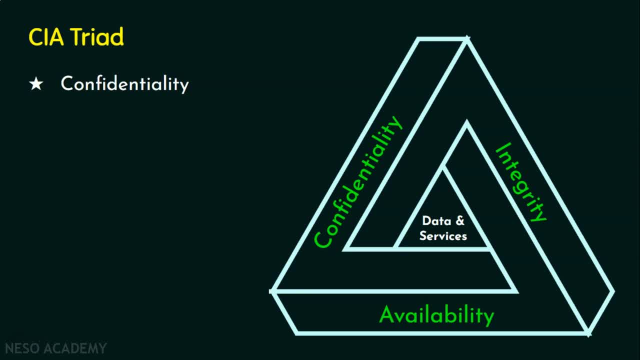 be able to understand what is the message that is being transmitted between the two parties, Between the sender and the receiver. this is exactly confidentiality. Let's come to the second key element in CIA triad, which is the integrity. I will just give you a formula. 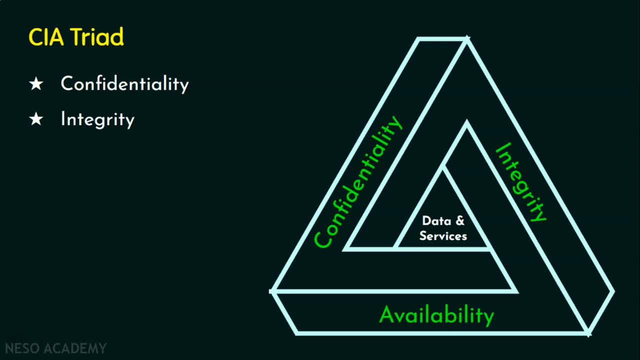 like this: Sent is equal to received. Whatever the sender is sending, the same message, only the receiver should receive. For example, if you are performing a banking transaction of 1000 rupees, obviously the transaction should involve only 1000 rupees. What if an attacker modifies this as 10,000 rupees? 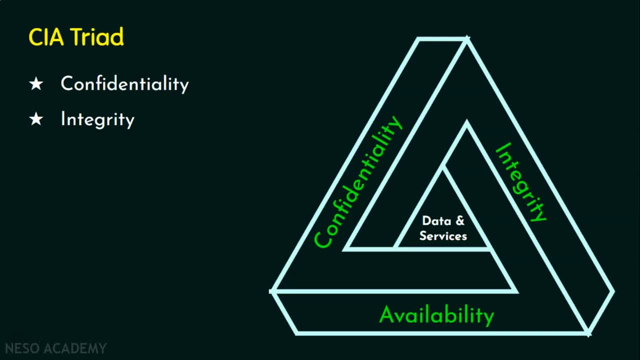 Let's see the modification of amount by the attacker. Let's assume the destination address or the destination account is given as the attacker's account. Just imagine this for an example. This may not be real and this may not be seeming to be a perfect example, but I wanted to make you to understand. 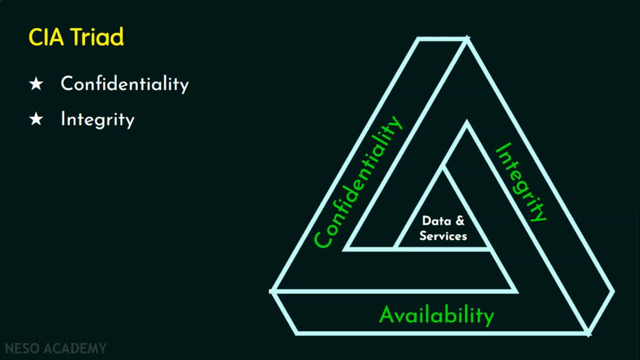 the severity of modification of message. I wanted to explain you what is integrity. So we don't want any modification of messages by the unauthorized people. Say you want to transfer some fun to your friend But unfortunately the fun is not being transmitted, or transferred to somebody else account, that is. 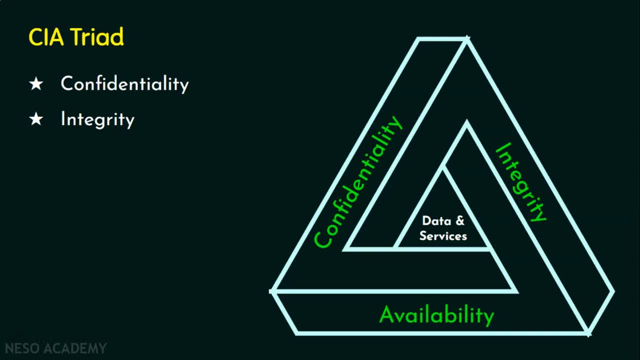 attacker's account. Obviously, this has happened because of the modification of the messages that is being transmitted between the sender and the receiver by the attackers. So this transaction should not be permitted by the system and the security system should be able to find out that this is not the message that was. 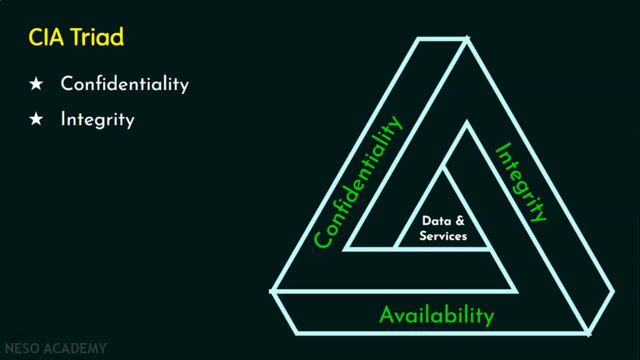 sent by the sender. In other words, the security system should ensure that this is not the transaction that was initiated by the sender. So integrity means we need to ensure that there is no modification of the message that is being transmitted. So, whatever the sender is sending that, only the receiver should. 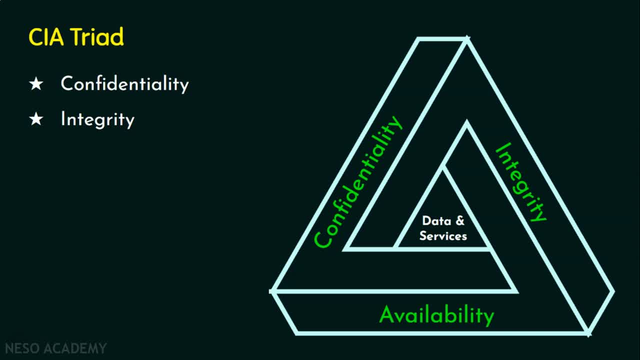 receive and if there is any modification in the message that is being transmitted, the system should be able to find out that and it should discard that message. So integrity is also one of the key terms of the CIA triad. and coming to the third key element, which is the availability, Availability means 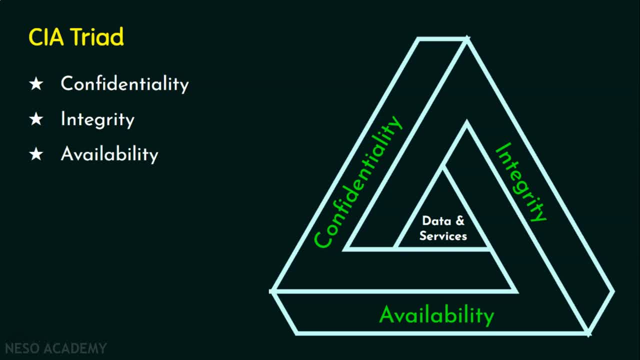 we need to ensure the timely and the reliable access to the system. Say, for example, if you are hitting googlecom, if you hit now, it will work. If you hit after one hour, it will work. If you hit after 10 days, it will work, because you trust that. 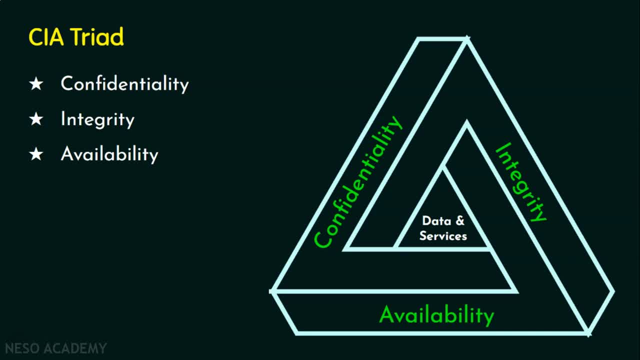 google server will be always available. At the same time, there may be many attacks that may be launched against googlecom server, but still, google server is a very secured one and google is able to provide its service to the customers or the users who access it without any flaws. So that's the power of a security. 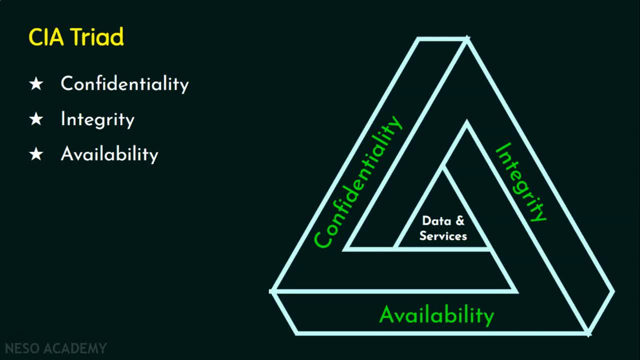 system. I will also provide you one more example. Imagine you have a bank account and you want to access your banking server. You are expecting the banking server to respond you with the requested data. What if an attacker has launched an attack on the banking server and disrupted the service? So 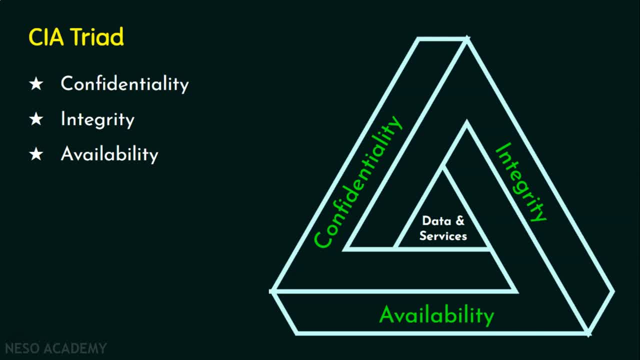 when you access the banking server, you are not getting the service that you are expecting. Obviously, we don't encourage that, because whenever we want a service, we expect the system to provide service to us, and this service should be a timely and a reliable service as well. There will be attackers always. 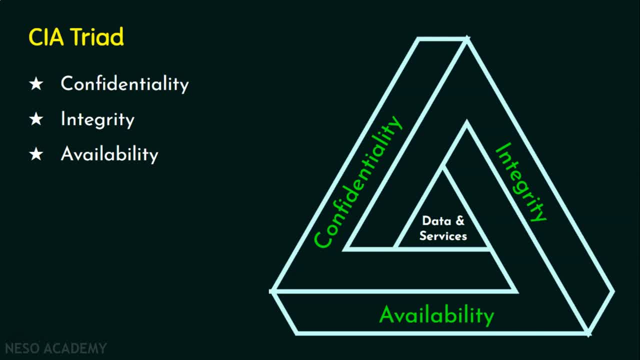 on the internet and our security system Is expected to provide security to the system and to the users. and whenever any attack is launched on the server, we expect the server should withstand that attack. It should still be able to provide access to the servers in the same way as it was in. 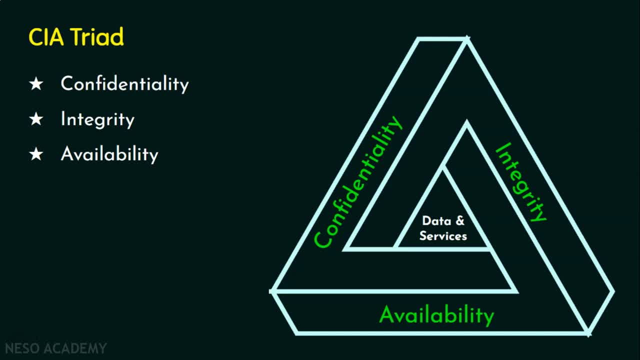 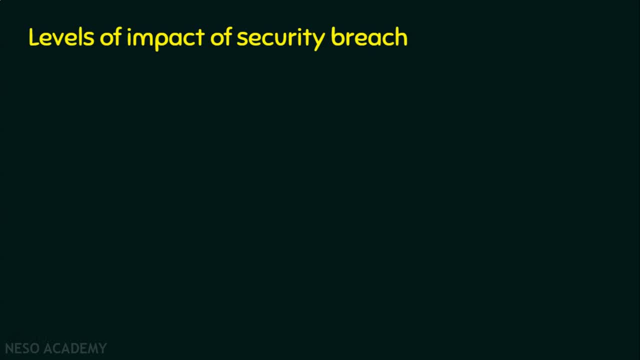 the perfect situation. and that's it about the CIA triad. Let's now navigate to the levels of impact of security breach. When there is a security breach in the organizational data, or to the server or to an individual. basically, there will be three levels of impact. 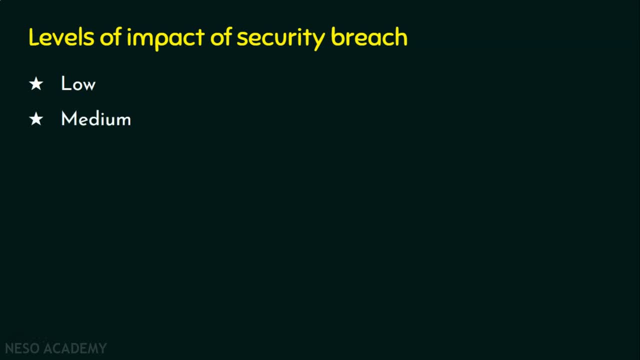 Number one is the low level impact, number two is the medium level impact and number three is the high level impact. We will see the various levels of impact of security breach one by one now. Firstly, we will focus on low level impact. If your 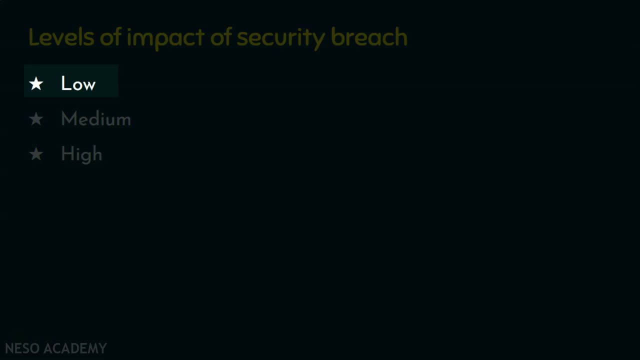 system is affected by some attacks and the low level impact means there is a limited adverse effect on organization's operation or organizational assets or individual. that is, the system is affected with minor harm or minor damage or, in terms of financial aspects, it is a minor financial loss If 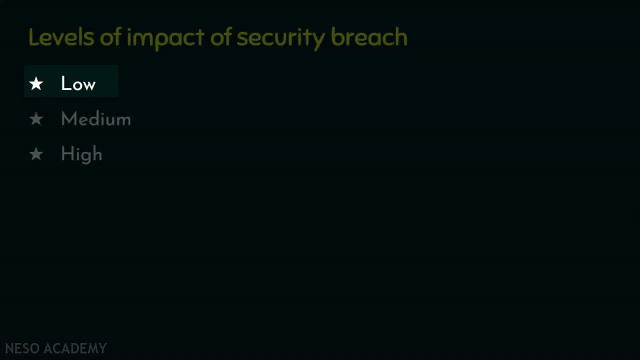 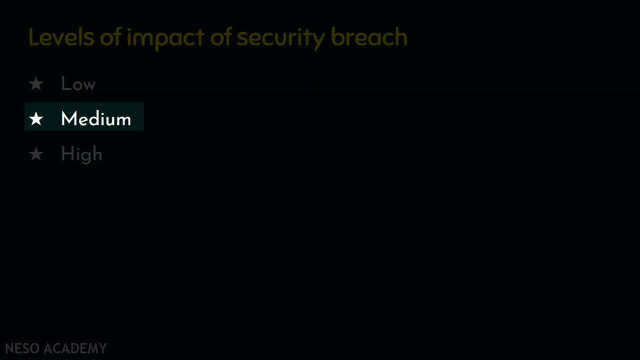 the effect of the attack is negligible, then it falls in the low level impact And coming to the next level of impact, which is the medium level of impact, it has a serious adverse effect on organizational operation or organizational assets, or even serious adverse effect on individual. So the loss may be a 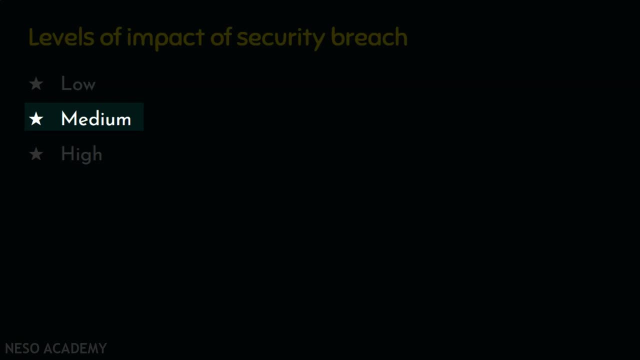 significant loss or a significant damage or a significant harm that is caused to the organization or to the individual. And this medium level of impact means the attack may be involving in the loss of life or even serious life-threatening issues. also, And coming to the final level of impact, which is 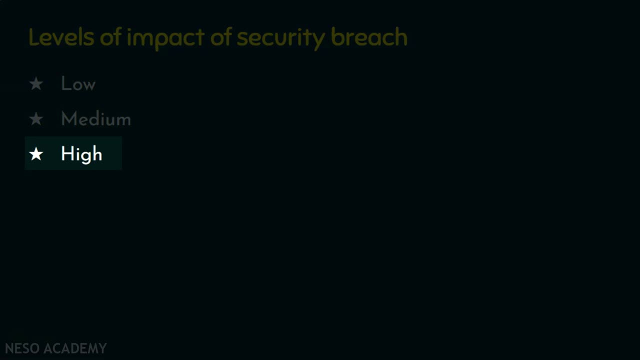 the high level impact. So when the medium itself is very dangerous, think about the high level impact. So everything is gone right. So the reputation, everything. High level impact of security breach means the organizational has catastrophic adverse effect. It means severe adverse effect on organizational. 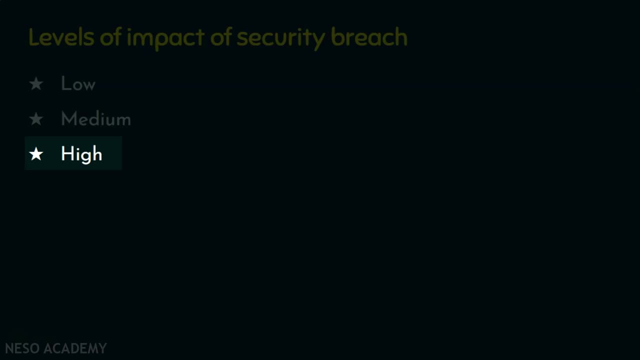 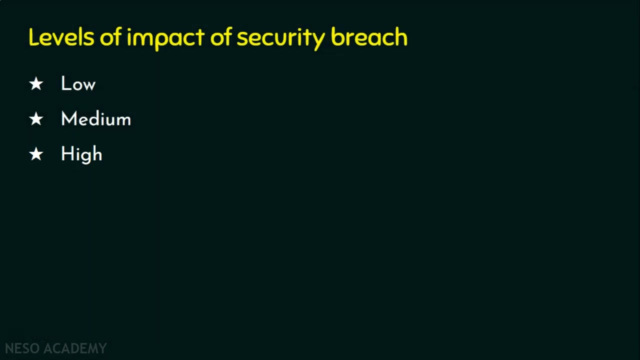 operations or organizational assets or individual, It is a complete disaster to the organization. So these are the three levels of impact of security breach, and this could be for an individual or for an organization, or for an organizational data, or for the information system or for any kind of stuff that really needs security. Before we step. 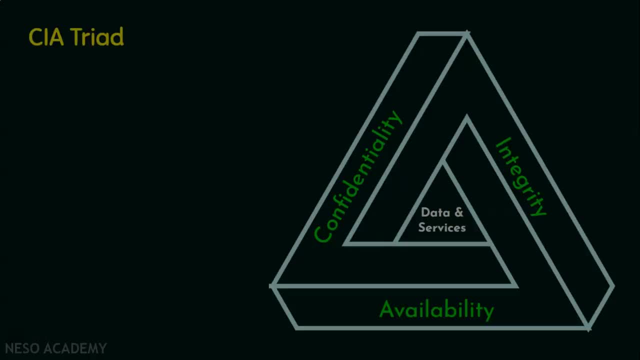 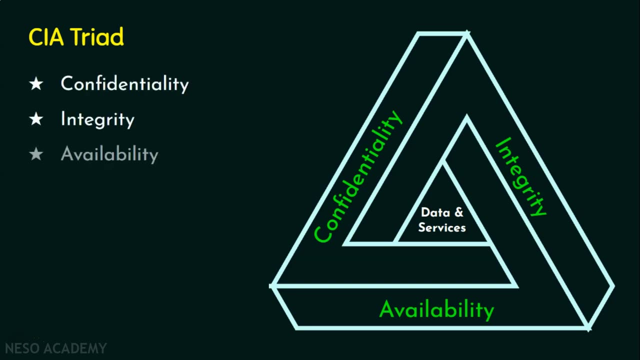 out. let's see the additional features of CIA triad. Basically, the CIA triad includes only three key elements: right, The confidentiality, the integrity and the availability. We also have two more additional elements, and the additional elements are number one, the authenticity, and number two. 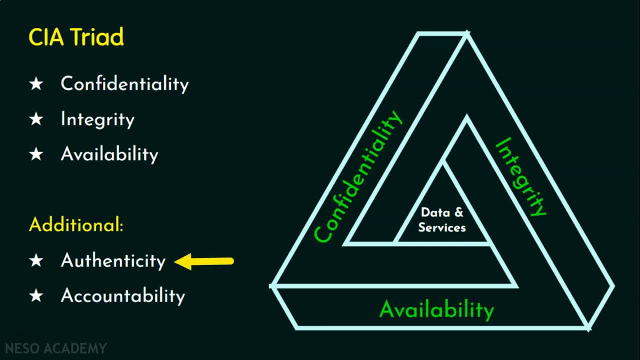 accountability. Authenticity is the property of being genuine and being able to verify the parties involved. Say, if the sender is going to send some message to the receiver. Say, if the receiver is receiving a message and the receiver should be able to verify that the message is from the right party. 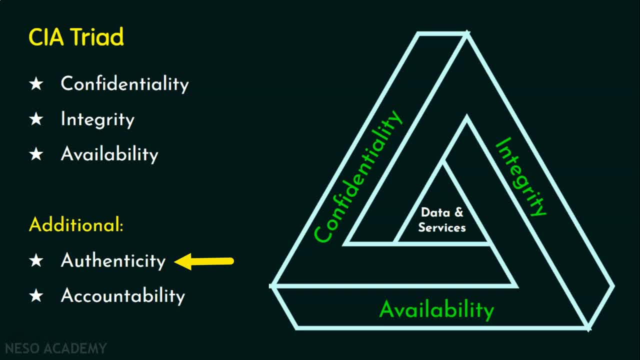 or the messages from the trusted source. We will call this property as authenticity. In other words, let's say you are accessing Google Drive. Suppose if you give a request from your browser as wwwgooglecom and you are expecting that your request is going to Google. 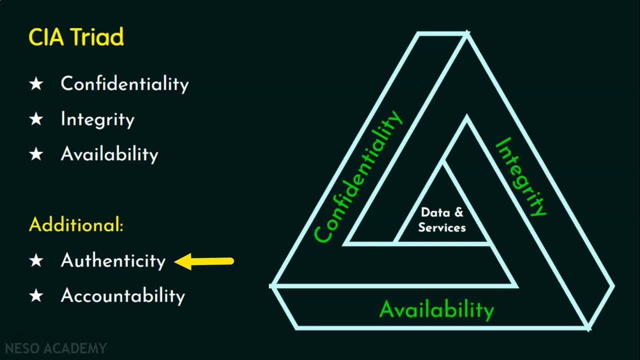 server and not any bogus server, right When the request is received by Google server and Google should be able to verify that it is from you. So this is we call as authentication, or authenticity. and coming to the next additional element, which is accountability, Say, for example, accountability is also. 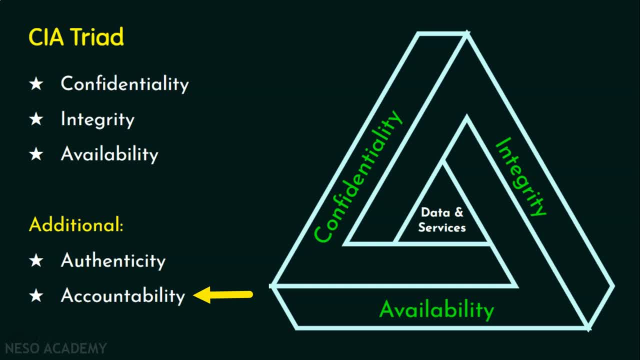 an essential part of an information security plan. It means every individual who works with an organization or who works with an information system should have specific responsibilities for information assurance. Every user who access the system has their own roles and responsibilities and, whatever the actions the users perform, the system should keep records of. 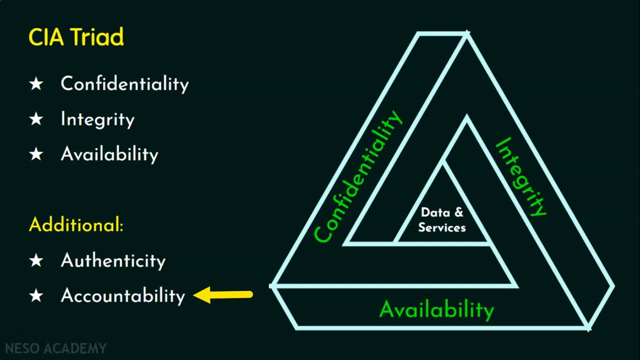 their activities. Why system should keep track of the activities? because later, if any attack is launched or if we find that something is suspicious, then the system should permit forensic analysis later to trace the security breaches. So in order to do that, we need to ensure that the system 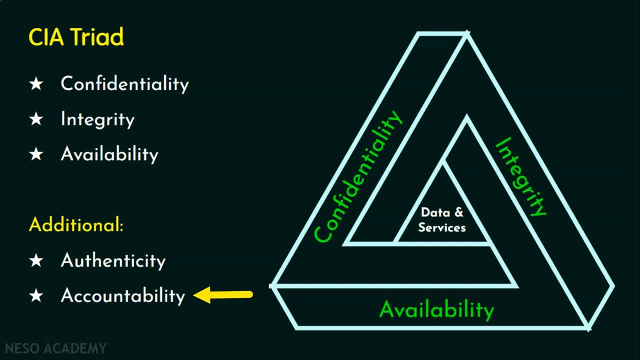 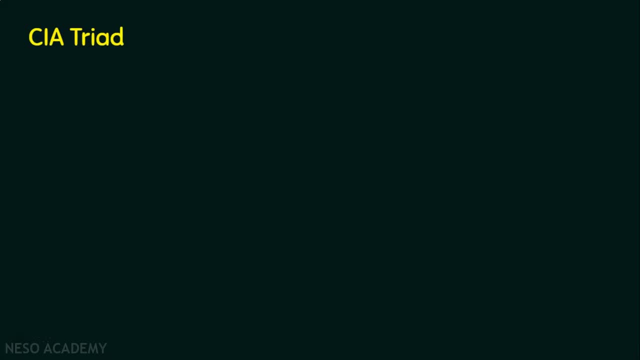 is accountable. Every user is given some responsibility and every user should access only to that level of privilege, or it must ensure that the users are not misusing their privileges. Let's see some real-time examples for confidentiality, integrity and availability. The first one we will see is confidentiality. 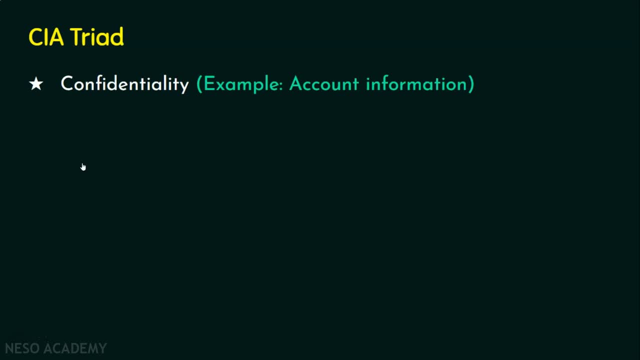 For example, the banking account information. Say, you have your mobile phone and you have your banking app in your mobile phone. You request some data from your banking server and from the banking server to your mobile phone or to your desktop, from where you are going to access the data. traffic must be encrypted. 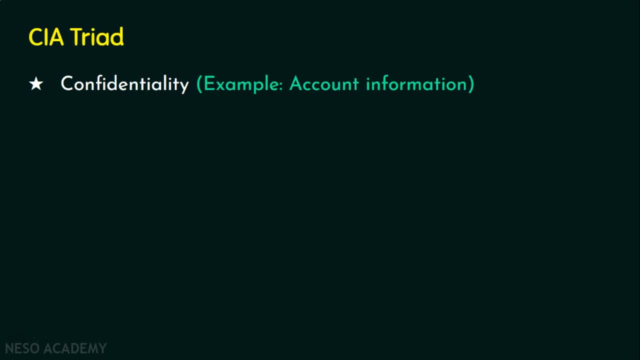 What if the data is not encrypted? Obviously there are chances for the attackers to see what information is being transferred between the sender and the receiver, So we don't encourage that should happen. So encryption is one of the ways we can achieve confidentiality. If the message is encrypted, accept the server. 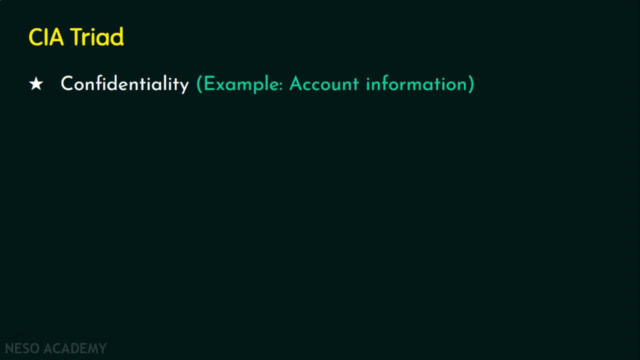 and you who are accessing the system. No one else can understand what it is, So the message must be encrypted. Encryption is one of the ways to achieve confidentiality. Coming to the second example, which is integrity, the patient's information Say, for example: 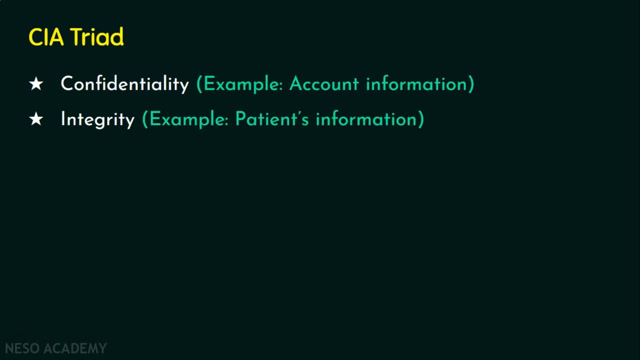 there is a hospital management system. Let's assume someone is having some disease and that person is installed with some sensors and the sensors are installed on his body. In this hospital management system, the doctor can be anywhere in the world and the patient can also be anywhere. 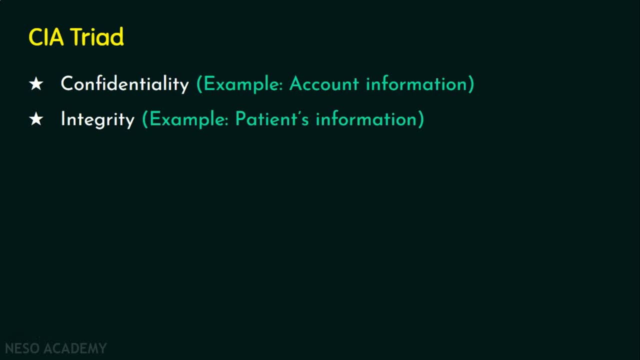 in the world The doctor and patient relationship can exist seamlessly because of the powerful internet connectivity and the IOT concepts- the internet of things. In this example, the patient is wearing a sensor and the patient or doctor need not be in person to do the medical treatment or to get the medical treatment. 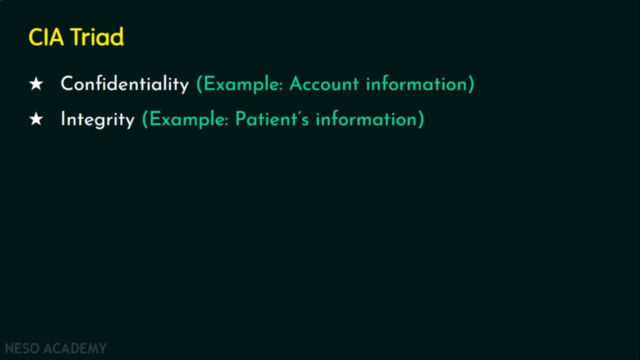 And what is the role of the sensor? You know the sensor is going to report the heartbeat rate periodically to the doctor via the servers. Let's assume the server is going to collect all the heartbeat information that is sent by the sensor. So obviously, whatever the sensor is sensing the heartbeat, 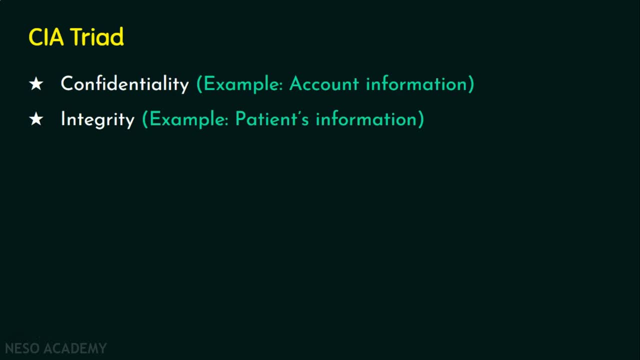 value that should be stored without any alteration in the server. only then the doctor will be able to provide right treatment to the patient. If the sensor is sensing the right value and the right value is sent to the server, but during the travel, if an attacker is modifying the value and if this modification 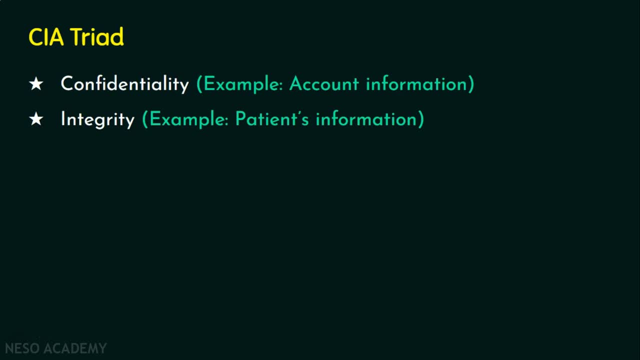 is stored in the server and when the doctor sees this modified value and is giving some treatment based on this, this could be a life-threatening issue also. It could even lead to lethality or fatality. Let's assume the heartbeat value that is sensed by the sensor. 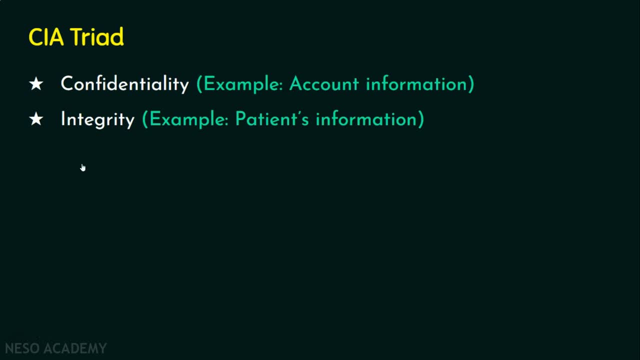 is 70, and this 70 is now being transmitted to the receiver, that is, the server. What if the attackers captures this packet and modifies it as 150?? So the treatment may go wrong, right? Because of this? so all patients information must be confidential and not only. 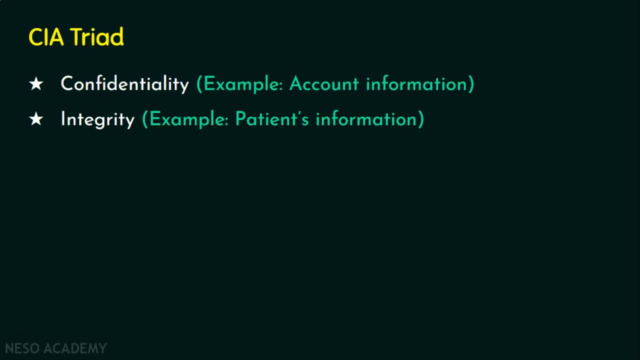 confidential. it should also have the property of integrity. So whatever the sender is sending, that only the receiver should receive, no modification should be permitted. So this is an example for integrity. and coming to the next one, the availability. example authentication service.